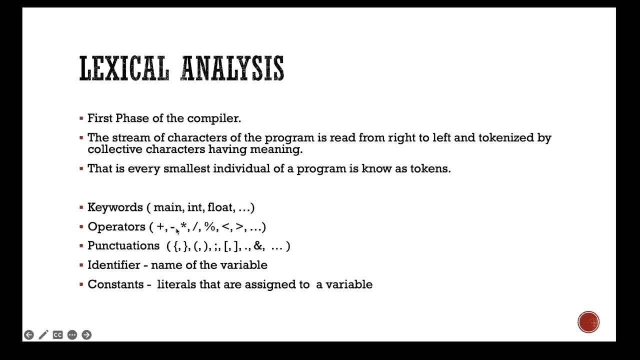 like to add. we have plus operator and the minus addition, multiplication, division and modulus, etc. And the punctuations are the symbols to end up the function. So the clannels, the open parenthesis, closed parenthesis and the semicolon, these things will be coming. 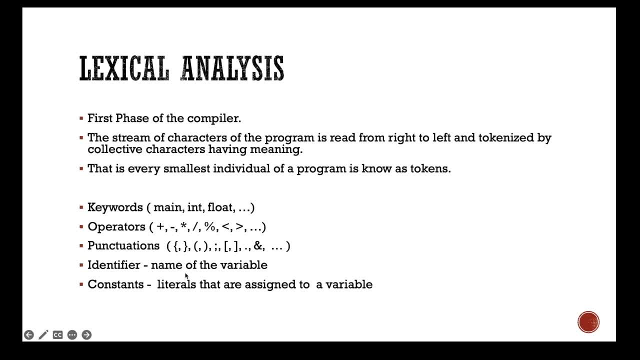 after punctuations. Identifiers are the value, like the, the number of characters, the number of letters, the name of the variable, array or number. Then you will be giving a variable, So that variable is identifier And the value you are giving for the variable is known as. 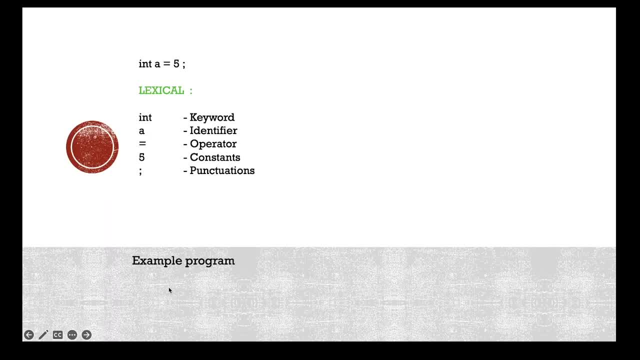 constants right. So now let us see an example quickly. So here I have taken line of code. So it is. here I have taken int. a is equal to 5.. So how it will be splitted in the lexical analysis and put into the symbol tables right, Int will be categorized into variables, So 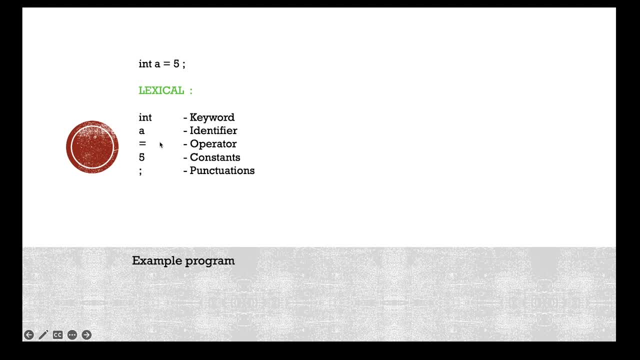 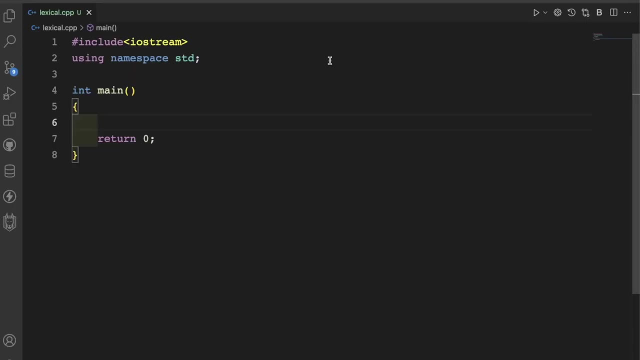 it is categorized into keyword, and a is identifier and equal to some operator, and 5 is a constant and semicolon is a punctuation. This is how we will be defining the lexical part. So fine, Now you are ready to go for the coding part. Okay, First let us input the record. 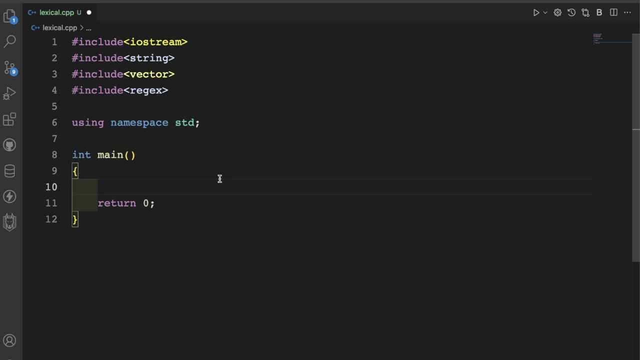 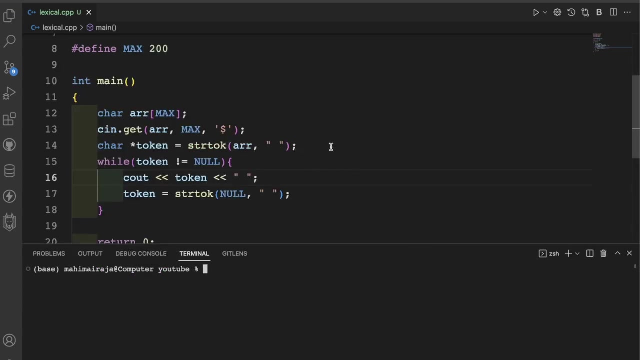 packages. So now let us get a multiply- multiply input from the users. Size of my array is 200, right, Okay, Okay, Let us split the program code using the string tokenization method. And now we will define a vector of keywords that are specified in the C++ language. So we just find the keywords. 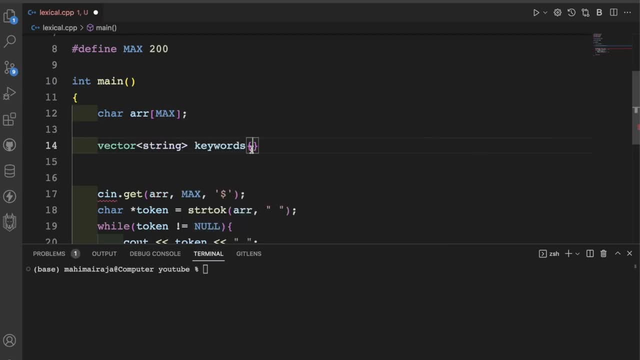 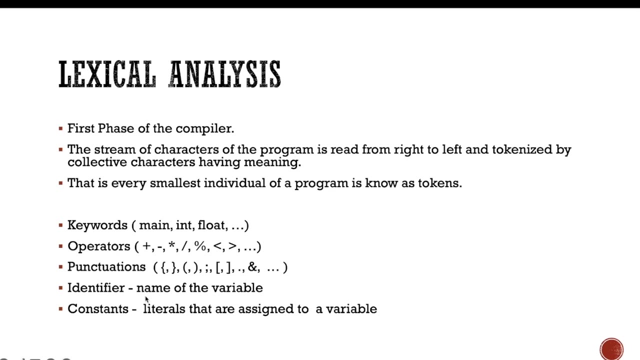 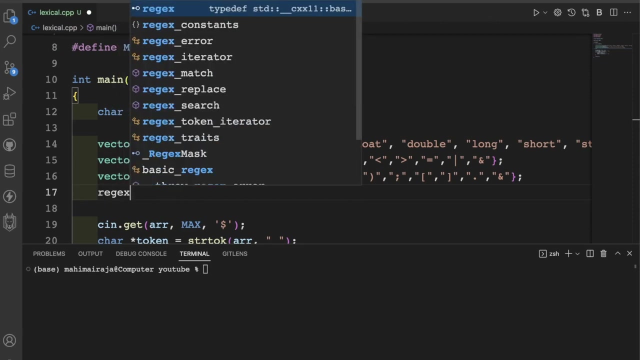 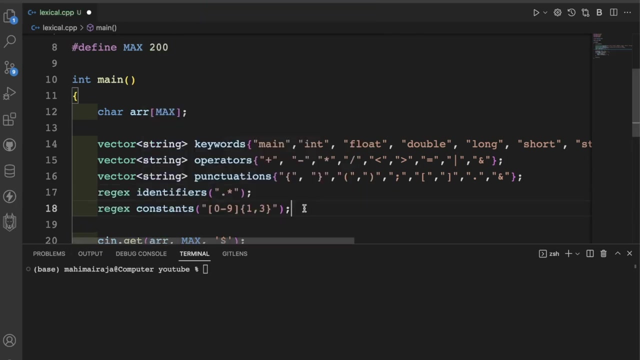 Similarly, we will also define the vectors for operators and punctuations. Now we will have left over in the identifier and constants. okay, So for now I will just use those functions- user rejects- to define the identifier constants. so now we will try to map it with the strings. 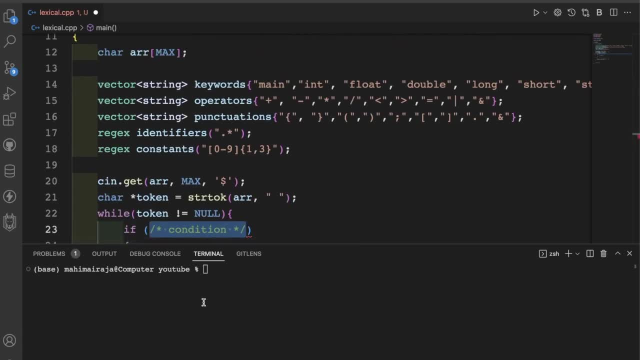 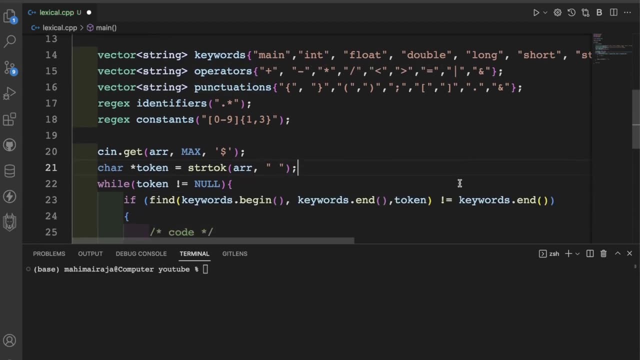 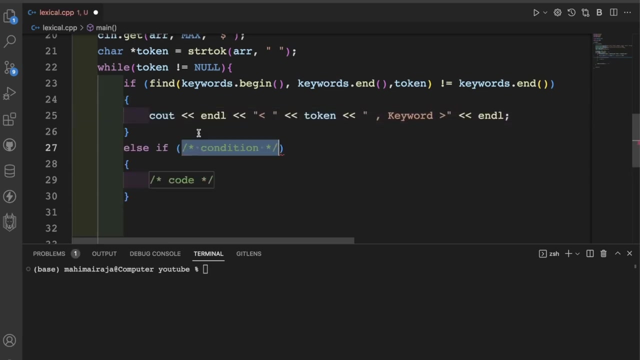 so the process is very simple. we are just taking a output like input of program code from the user and we will just try to compare with each element in this keyword. so if you find it, I will just print the output. now we will write the condition for the operators.